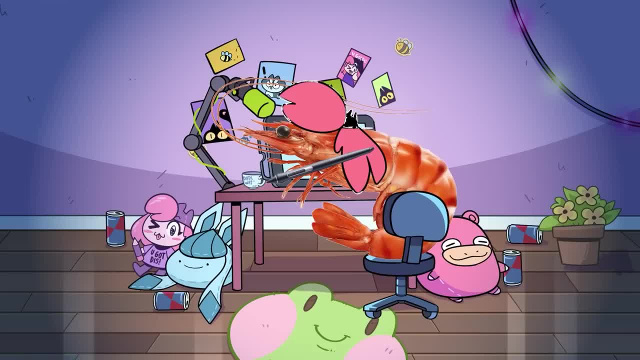 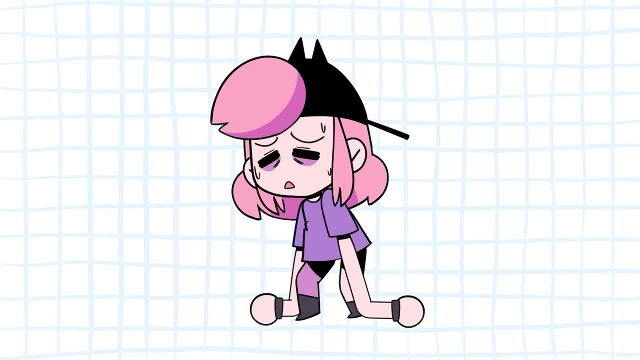 go outside. Life's too short to be shrimp posing in my art cave And to animate life you kinda have to experience life yourself. I usually don't like carrying laptops because they're way too heavy for my flimsy wrists. Lenovo has slim and lightweight designs that start at 3.7 pounds, saving my traps. 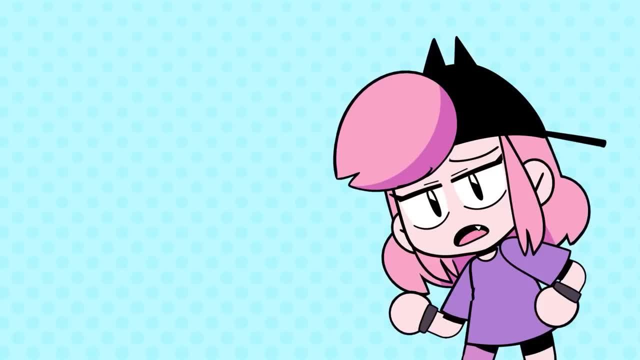 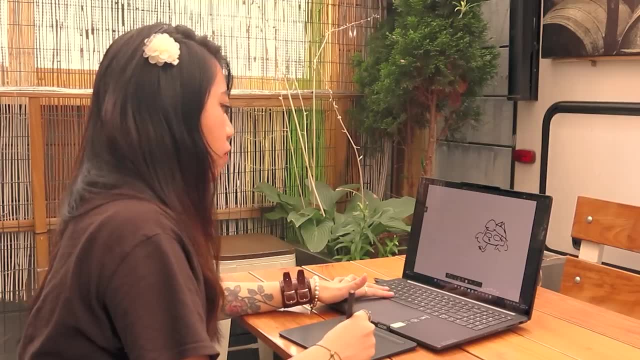 from being in the worst condition they've ever been. That way I can leave my skin dry And I don't need to worry too much about finding an outlet at my local cafe. Here I'm usually just coming up with topics that I would like to talk about. I'm usually sketching. 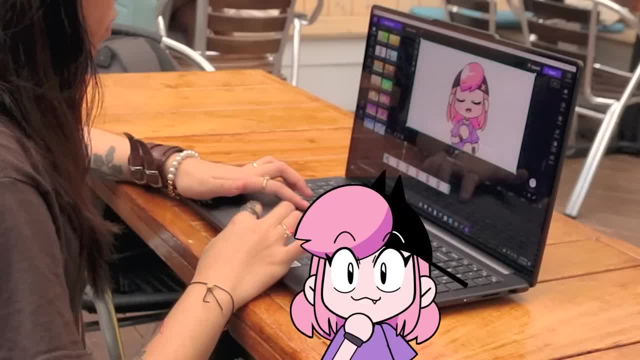 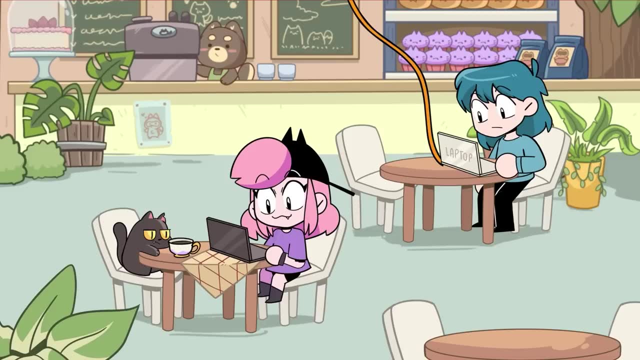 while I'm writing out my thought process, And since I'm a beginner, I'm going to go ahead and do some sketchbook, 300 pens and a highlighter at home. Now back to coming up with an idea. The Lenovo Slim Pro 9i comes with some awesome tools, like the Microsoft Journal app, where I 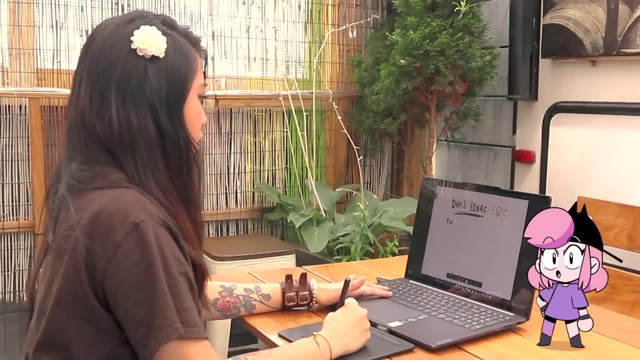 can do quick doodles in, But wait, there's more. I've been trying to get out of the art cave more so. the Lenovo Slim Pro 9i works great with its 9 hour battery life, Which means that I don't need to. 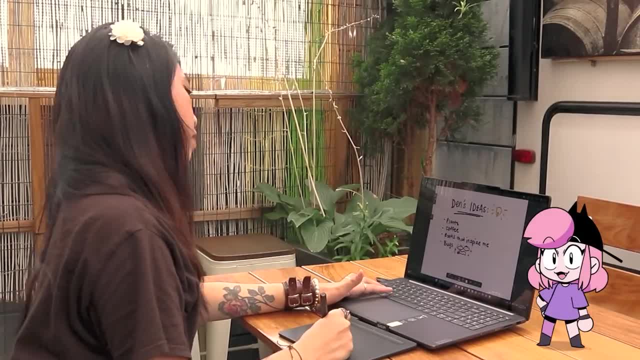 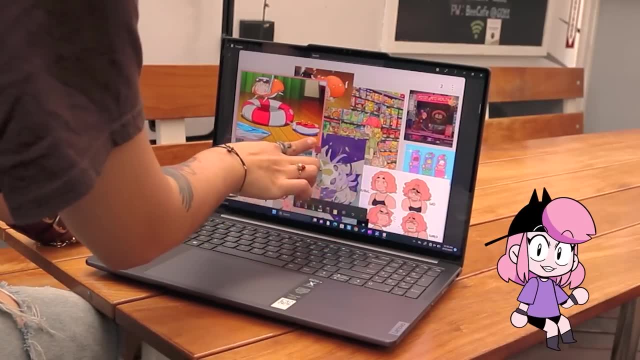 worry too much, And since I'm a very visual person and words are hard, I like to put my ideas down on the journal app, where I make a little mood board of inspiration using images and art styles that I clip from Pinterest, Google, along with TV shows and movies I've watched Here. 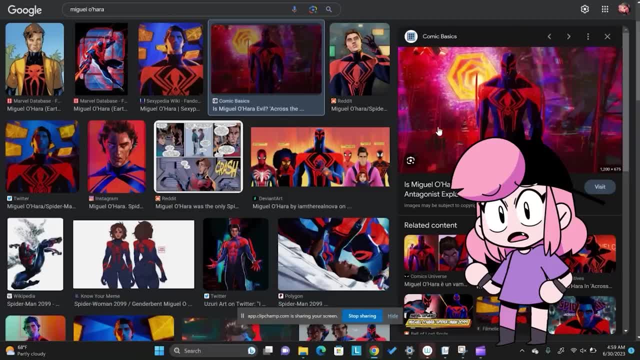 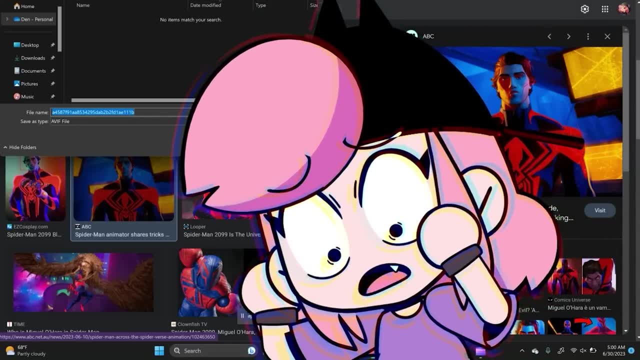 I'm using the snipping tool because I cannot, for the love of pasta, figure out why we, as a civilization, would create file types that would make saving pictures way more difficult than what it's supposed to be Like. why, What's the point? Anyways, once I have an idea that I'm 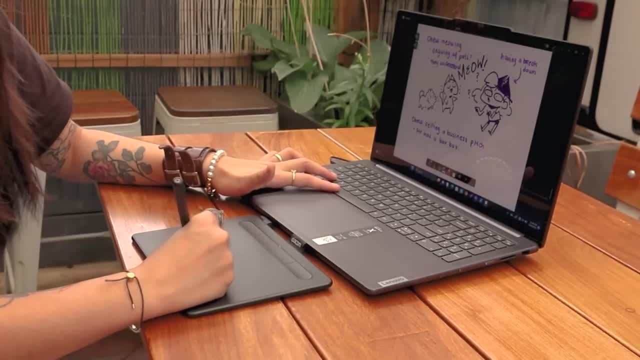 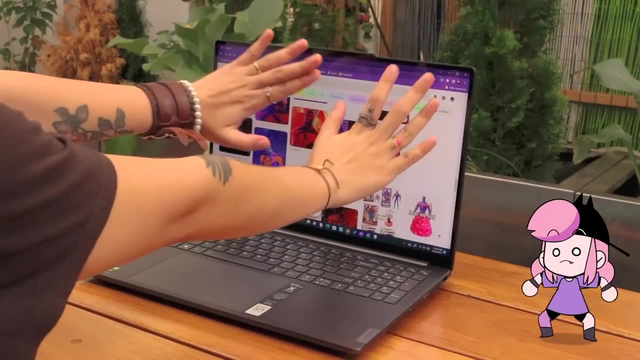 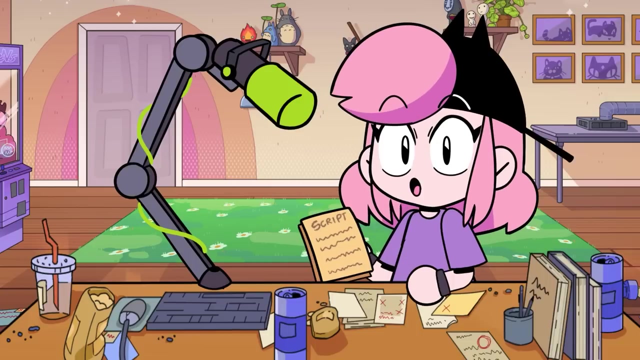 excited about, I start writing bullet points. These bullet points are topics with an idea that I find interesting and might want to expand on. This is when I record my script. Animating to a pre-recorded audio is easier for me, so I have an idea on how long the video is. 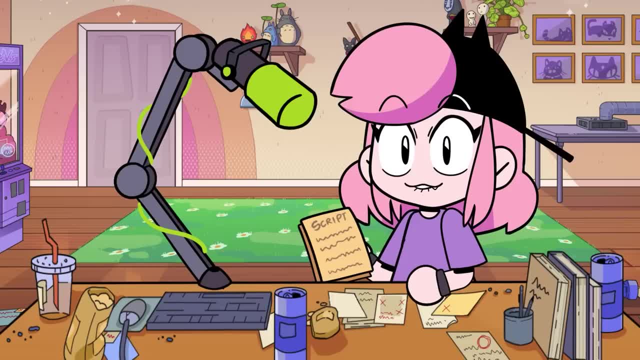 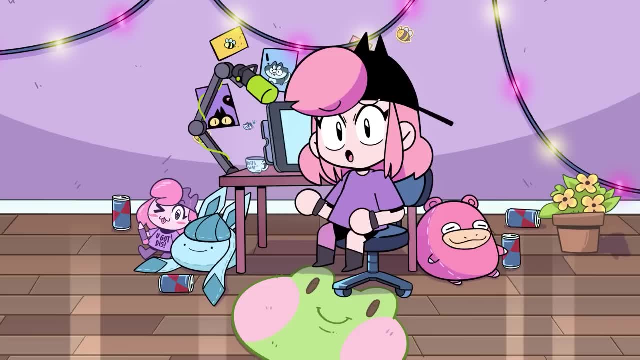 and so I'm not spending too much time drawing a frame that you'll only see for 2 seconds. I'mma be real with you- not my favorite part. I'm not fond of hearing my voice and hearing myself pronounce words a billion times over, but you just gotta believe and learn to love your voice. 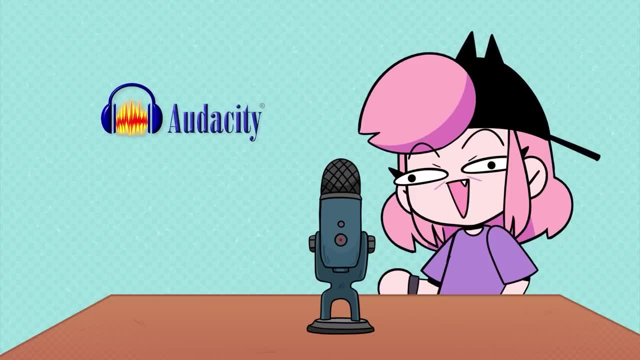 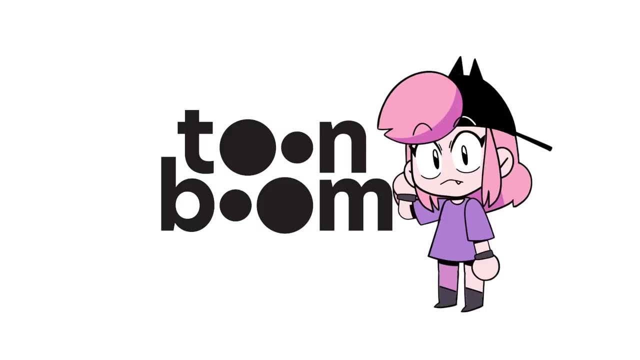 To record my audio, I use a program called Audacity. I also use voice mods, as I voice all my characters so I can sound like this. And after I'm done talking to myself, it's time to storyboard. For this I use Toon Boom Harmony, But I know it gets a little pricey. 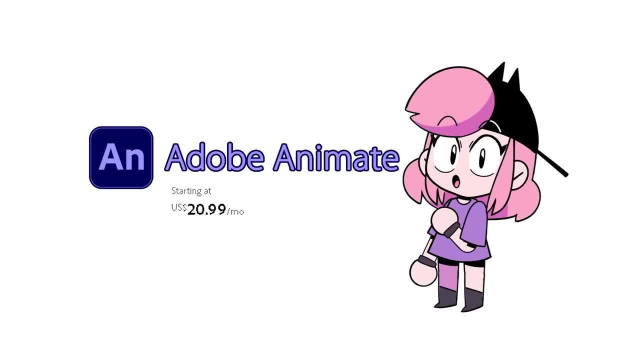 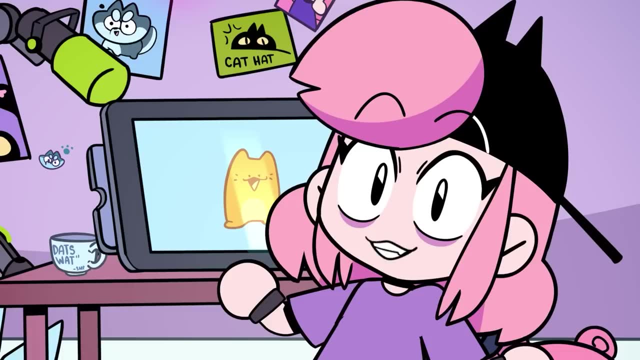 Animate CC is a cheaper option which I started with And, if you wanna try it out, the Lenovo Slim Pro 9i comes with a complimentary 2 months of the Adobe Suite. For me, storyboarding comes in many phases: The super sketchy stick figures. This is when I just lay out which characters 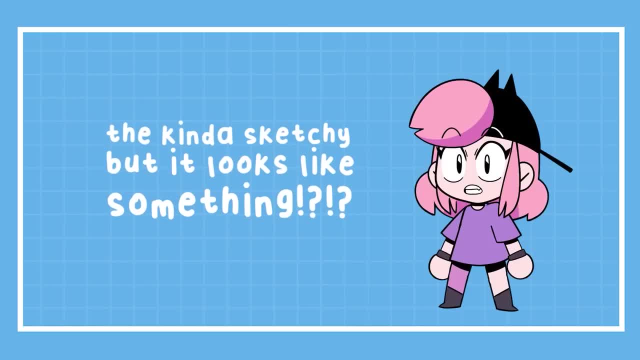 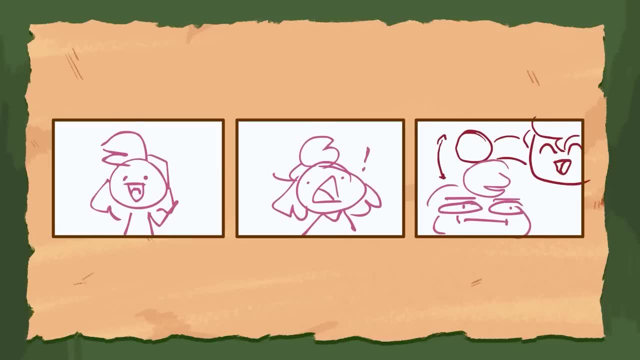 would be in the shot and the most basic ideas. The kinda sketchy, but it looks like something. This is when I try to capture the basic poses and expressions of the characters- Still super sketchy, though. After this I try to get the timing and the movement as 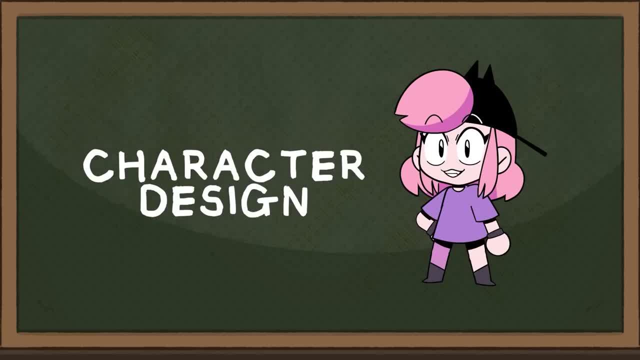 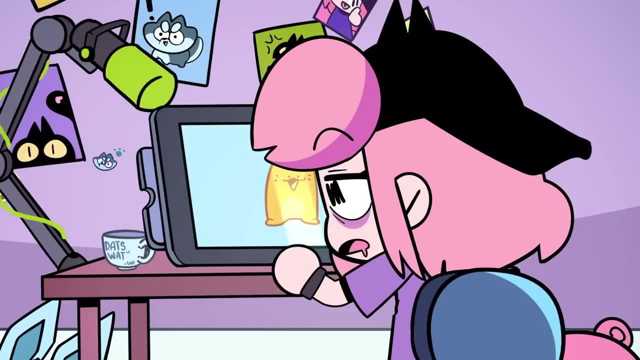 close as possible to the way I want it. before the cleanup: Character design: This usually goes before storyboarding, but since I'm working on a quick turnaround like YouTube, I'm usually down to the wire for a lot of these things, So let's speedrun character design. 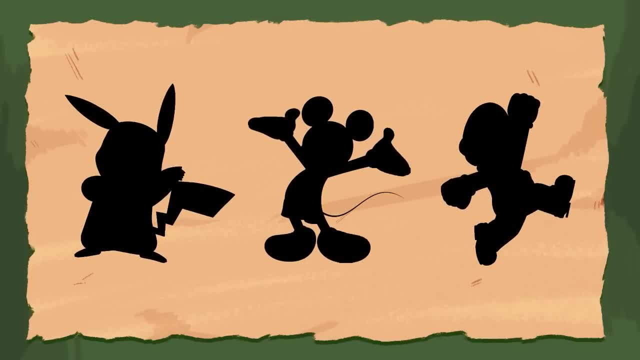 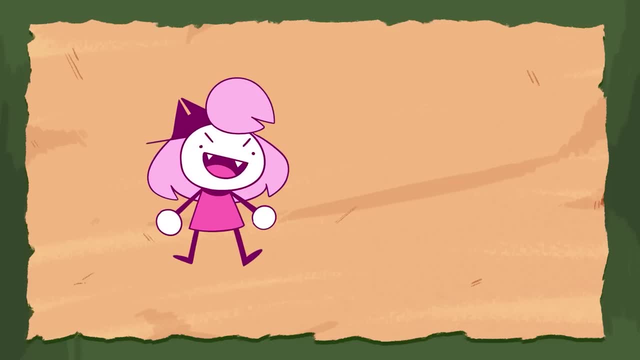 Make sure you focus on recognizable silhouettes that make your characters stand out. Make each character distinct from one another. If one is tall, make the other one short. If one is big, make the other one small. If one is pink, make the other one blue. 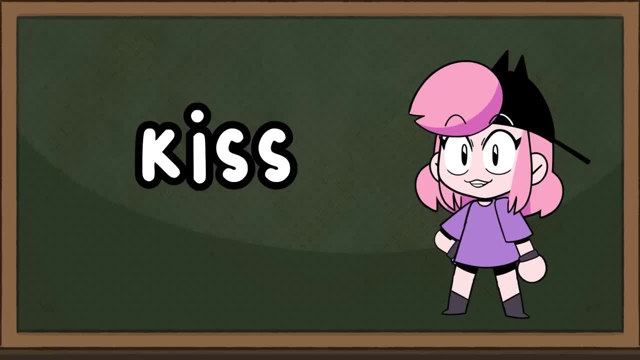 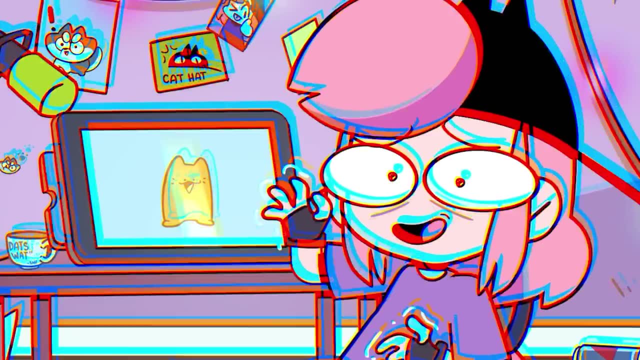 If you're making something for animation, always remember KISS, Keep it super simple, Because having to animate a super complex character when you're on a solo mission is just asking for carpal tunnels at an early age. Most lovable characters are very simple in color and design anyways, But if you're having an art 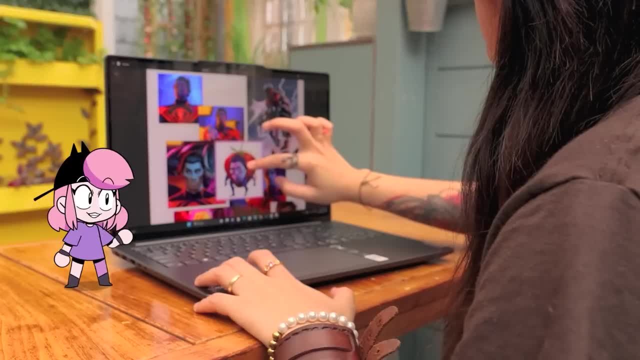 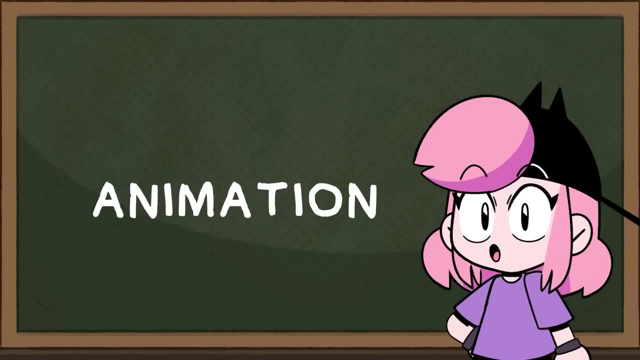 block at this part. you can always grab inspiration from your favorite characters, cool shapes, designs and even colors. Pick and choose what parts of the designs you like most. Animation: Animation is the heaviest of the workload. You can animate either. 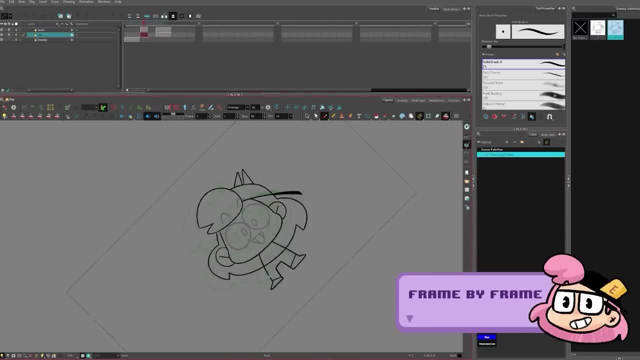 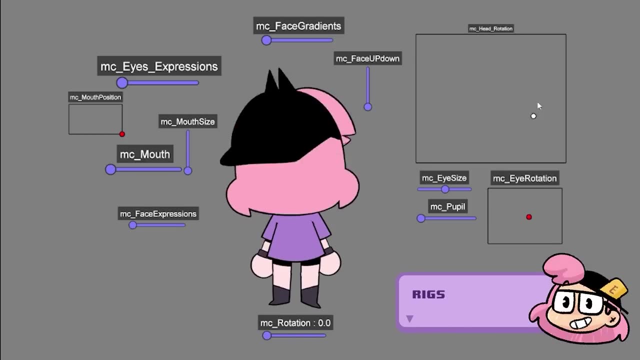 frame by frame or with rigs. Frame by frame usually requires you to draw and color each frame of the animation, Or you can use rigs for your animation, which is what I'm currently using. Rigs allow you to make kind of a puppet skeleton out of your character, so you don't have to redraw them over. 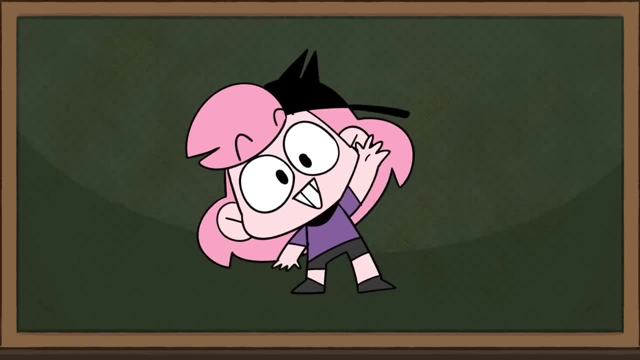 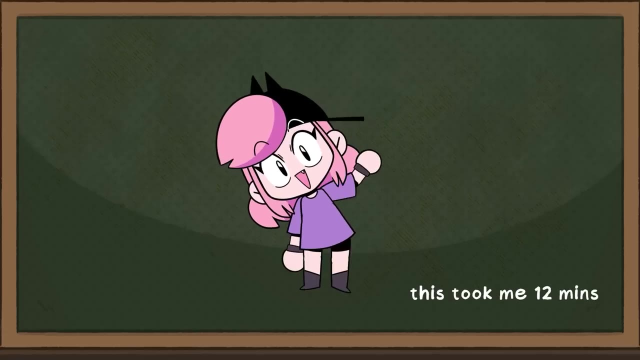 and over again The pros and the cons. Frame by frame animation allows you to animate with fluidity or more dynamic poses, But it does take a lot of time. Rigs are very limited in poses and can sometimes look very stiff, But it saves you a lot of time, Saves me a lot of time. You kinda just 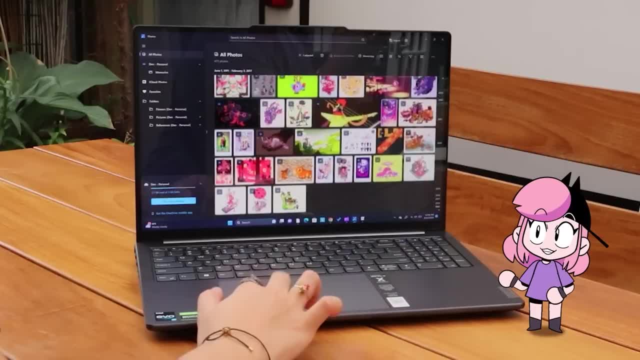 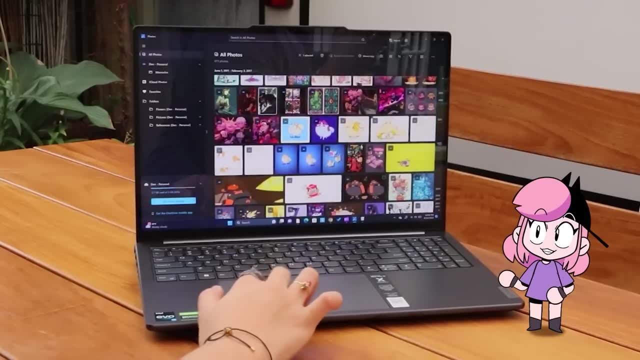 have to pick which one's the best for you. Throughout this process, I use a lot of references From Pinterest: movies, animations, pictures from life- Anything I feel like would fit the feel of the animation. References help you build your characters From using different. 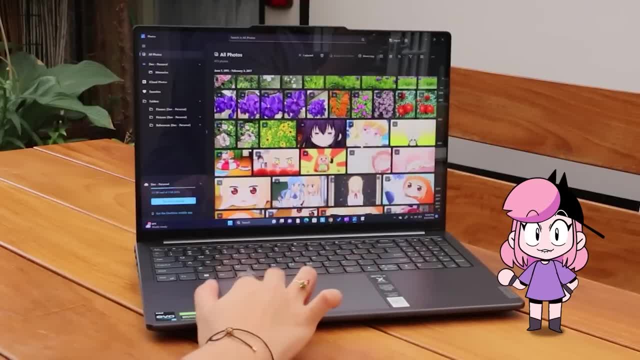 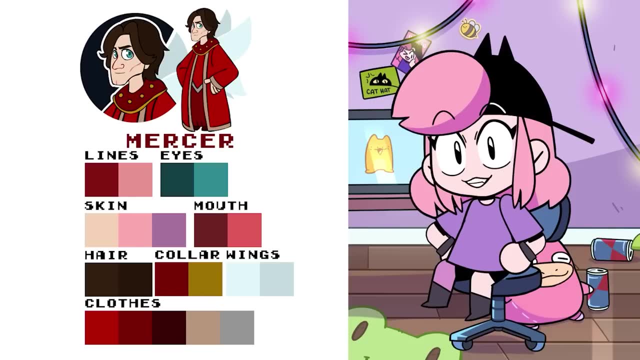 art styles for inspiration, ideas for their clothing, guidance for poses, movements, colors and so much more. I usually try to get a rough idea of the colors I want to use before animating, Just so I don't have to recolor after the fact. But also, I can't tell you. 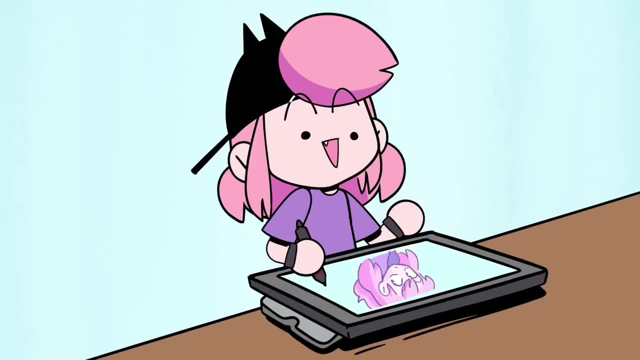 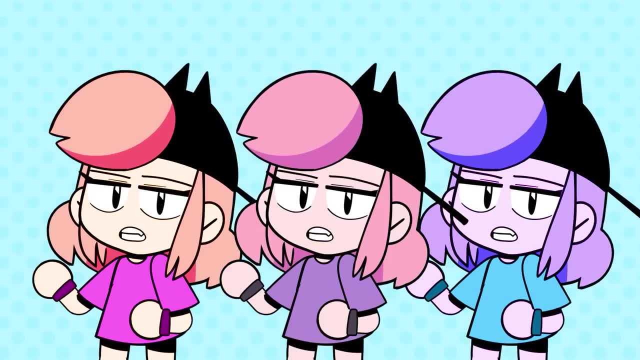 how many times I'm drawing, coloring and rendering a video and it looks all pretty on my screen And then after I upload, I realize I just colored my animation- the most heinous, obnoxious, sorry excuse of a color. But Lenovo got it figured out. The Slim Pro 9i has 3K mini. 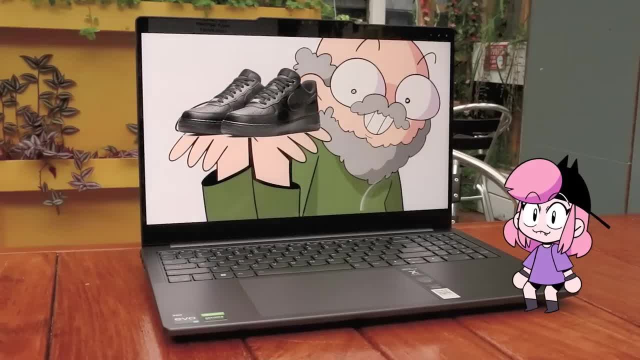 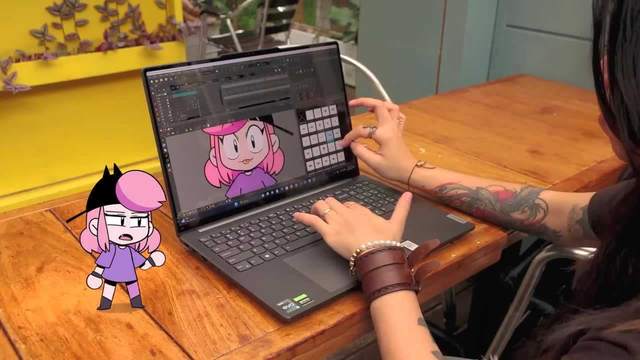 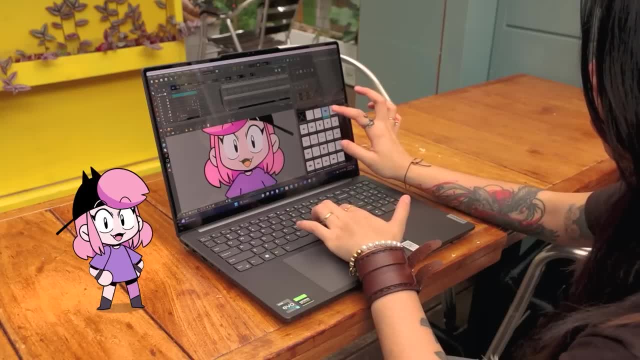 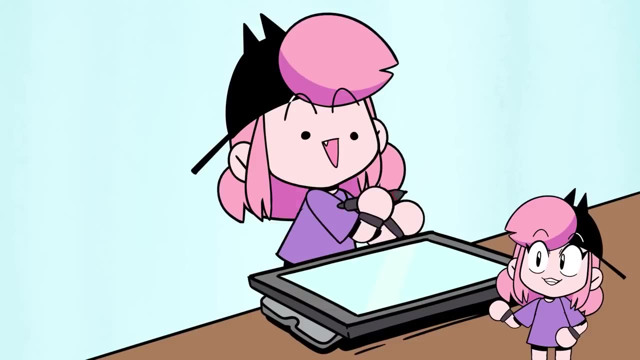 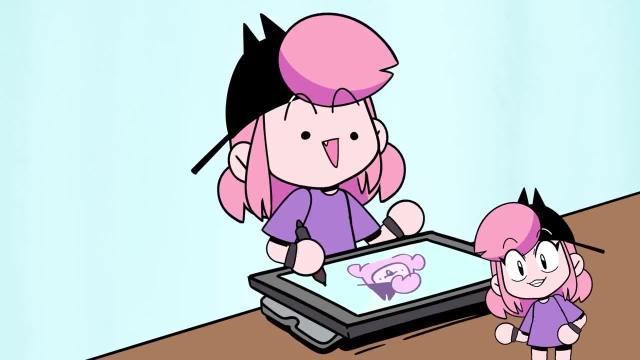 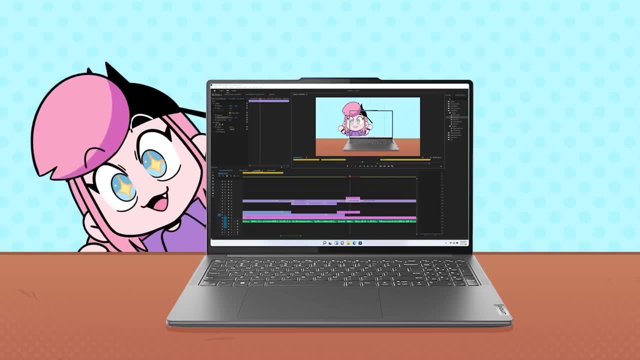 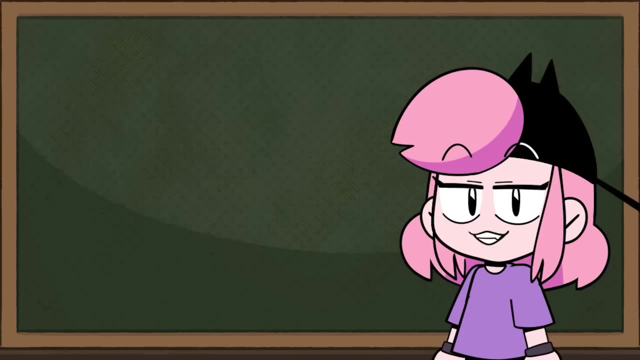 coloring and shading. on the other hand, you can do in batches. Doing these in batches makes it easier, so you're not jumping around tasks. Are we done yet Editing? To edit, I used Premiere Pro, which can be a little complex, But if you're looking for something easy to learn and free, 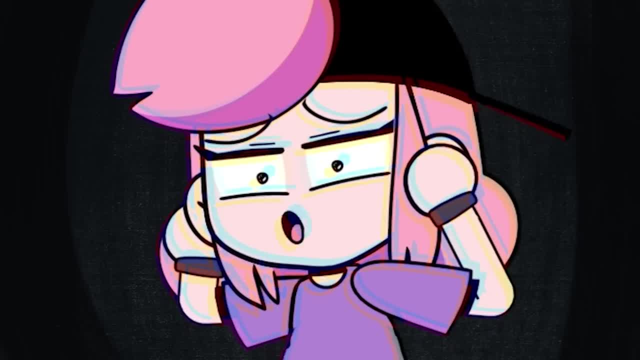 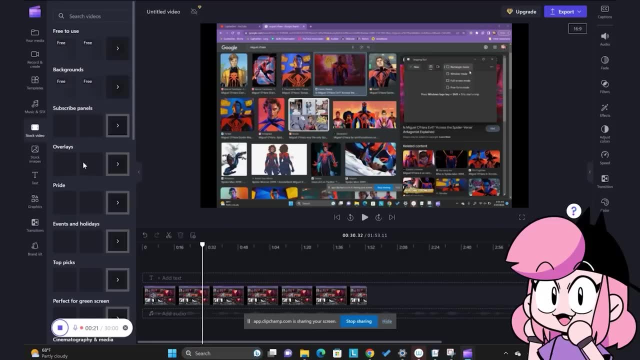 I've been trying out Microsoft's editing app called Clipchamp, And where was this when I was starting out? I actually use Clipchamp to record the on-screen process you see in this video, And I like the fact that there are stock images, stock video, video templates and music, which makes it.